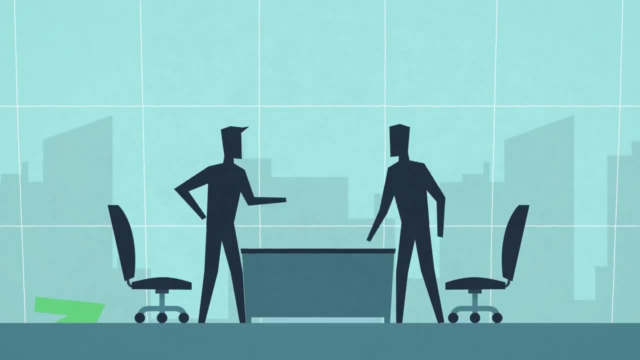 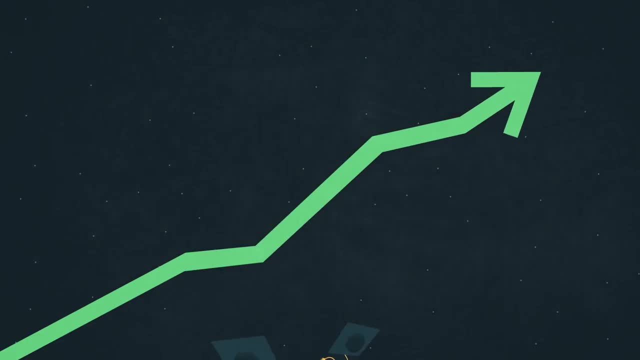 level of growth is possible, but it will require policies that encourage people to rejoin the workforce, and policies that spur more investment in education and the tools that help make workers more productive. 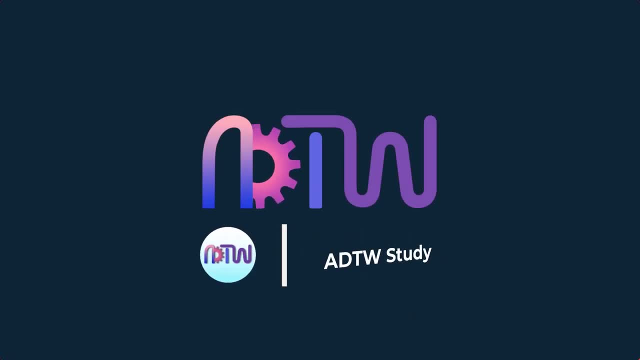 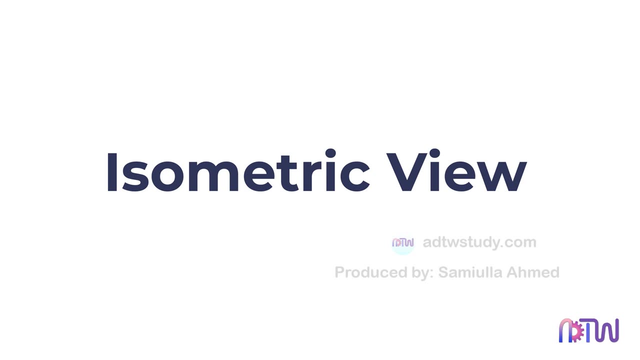 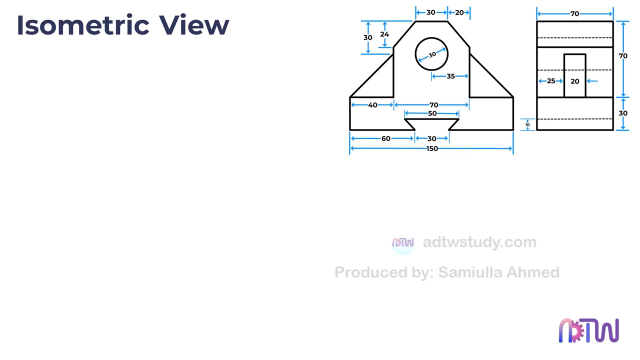 Isometric view. In this video we will learn how to construct an isometric view using orthographic projections. This is our seventh video on the topic. These are the orthographic projection of the object. To construct the isometric view or 3D view of the object we first need to create. 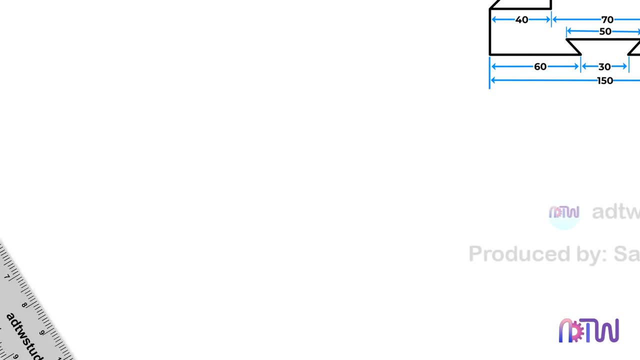 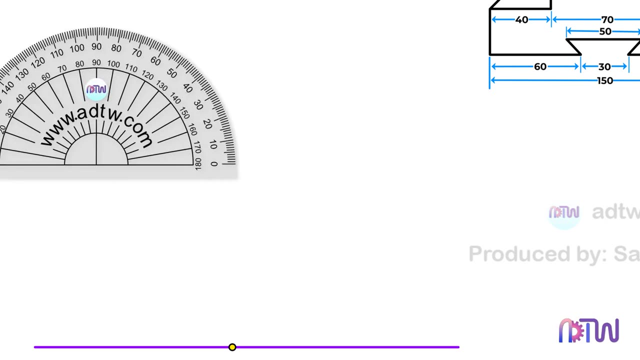 the isometric axis. To do this, take a ruler and draw a horizontal line, Then mark a center point on this line. Next, take a protractor and mark 30 degrees on both sides of the center point, as well as 90 degrees. Draw lines passing through these points from the center point. 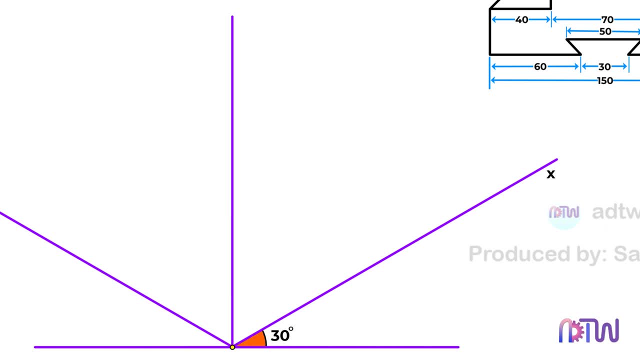 The line passing through the 30-degree mark will be the x-axis, the line passing through the 90-degree mark will be the y-axis and the remaining line will be the z-axis. With these three isometric axes in place, we can now construct the isometric 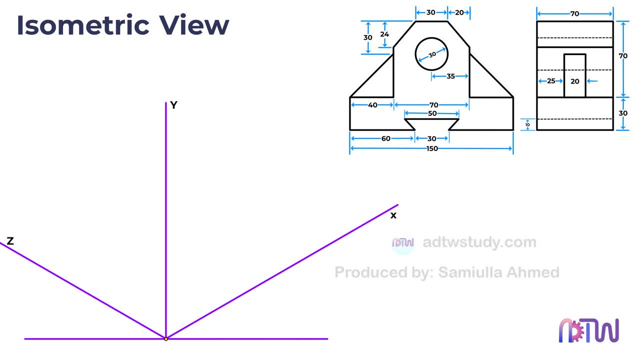 view of the object. Next, we need to decide whether to draw the front view in the x-y plane or the y-z plane. It's important to remember that the front view should only be drawn in these two planes and never in the x-z plane. The top view of the object is always drawn in the x-z plane. 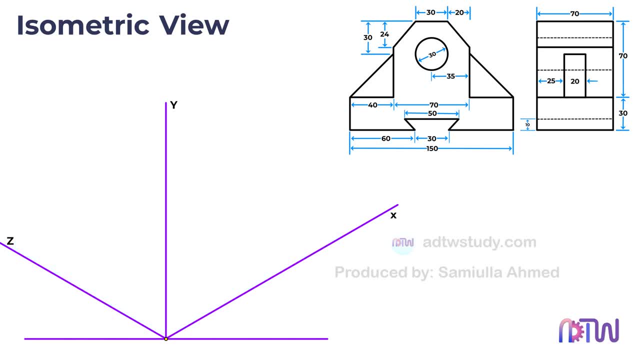 so that's another key point to keep in mind. In this video, we will be utilizing the first angle method to solve the problem. The figure on the left-hand side represents the front view, while the figure on the right-hand side represents the left-hand side.